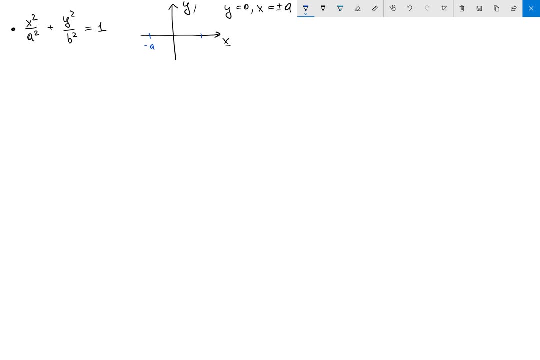 direction. I will have intersection minus a and a and my ellipse in the same way. intersection with y-axis is going to be minus b, b, and I will have this shape. Okay, it's not perfect one, Let's do another one. Another one is a parabola and in this case let's say I have x equals a, y squared and graph for this one is going to be a little bit more simpler. I will have the same. 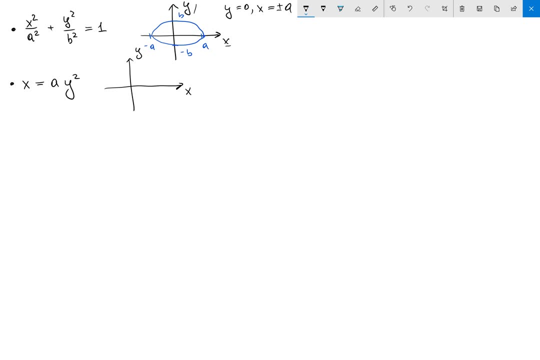 xy-axis and my graph looks something like this. It's going to be like just parabola in this direction. Okay, and my third equation is a hyperbola. And for hyperbola, I have x square over a square, minus y square over b, square equals to one, And for this hyperbola, the corresponding graph, the first thing I can see if I will set. 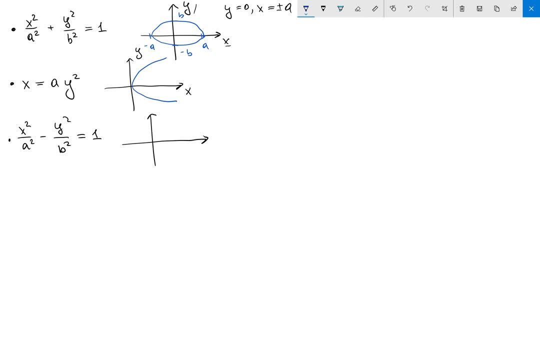 y equals to zero, I will find the same way that my a changes from minus a to a. but if I will get x equals to zero, I will have that y is going to be a imaginary number. so in terms of graph it looks like that my hyperbola gonna looks. 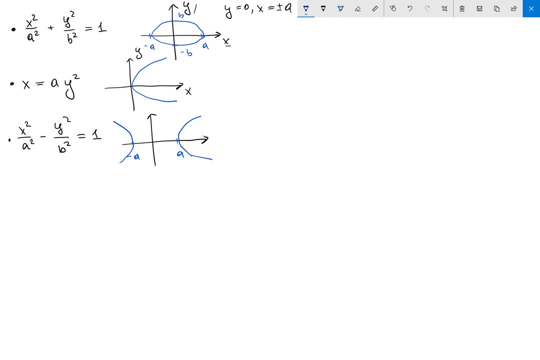 like this. okay, so while this like curves are actually going to be the same curve, the first like geometric intuition that if I have an ellipse, for the ellipse I have two points, it's called like focus of these two points and that's why ellipse- actually a circle is going to be an ellipse when all this focus points. 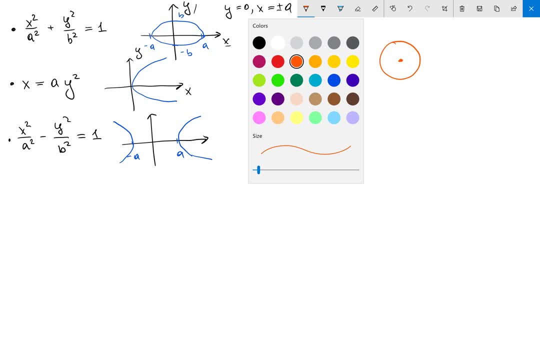 are going to be the same point, so I can think about my ellipse. in this case, how can we gonna get a parabola? I have my coordinate system, I have my parab, my ellipse, with two points. so what I'm going to do, I'm going to move my ellipse first to the right and I will have the 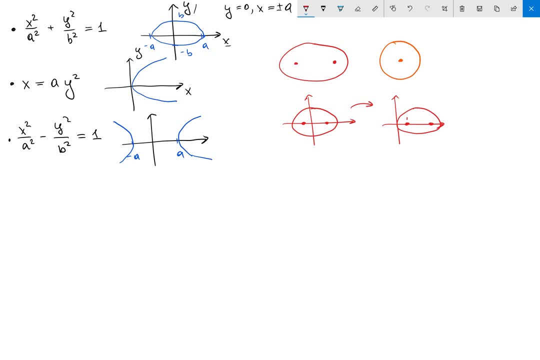 this shape and let's say I have a focus 1 and focus 2 and what I'm going to do with my next transformation? I will send focus 2 to infinity and then I will send focus 2 to infinity. I will get my desired parabola so we can. 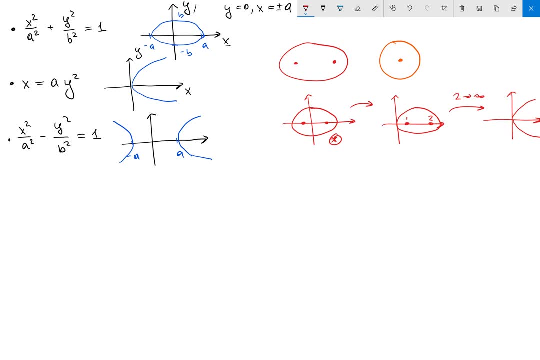 see that my parabola is going to be the same as the previous parabola, so we can see that how we actually move from an ellipse to parabola. so we just send our 2 to infinity and what we can do is like this infinity is so weird is that we can. 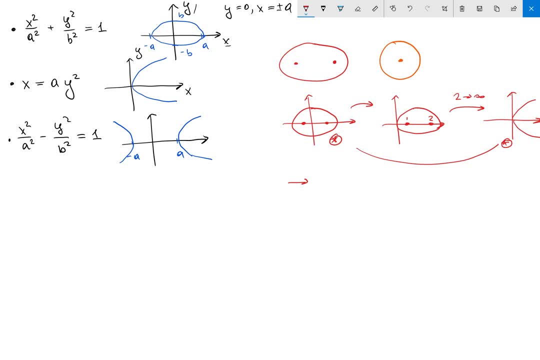 send back our 2 from infinity to 0. but what we're going to do, we're going to send it not from, like this direction, positive x-axis- but we're going to come back to 0 from other direction. so if we're going to come back from 0, 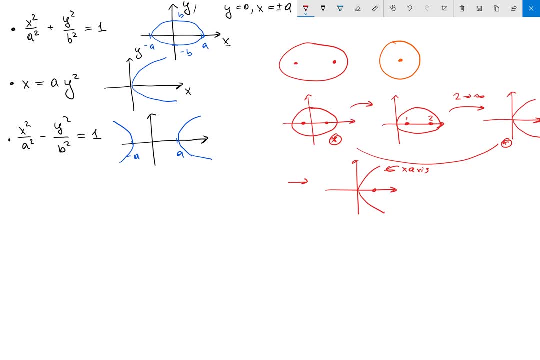 to other direction. this our one focus and we're going to come back from other direction. we're going to get our second focus and you can see that we move. we got a hyperbola, so we move from one an ellipse, to parabola, to hyperbola, just by. 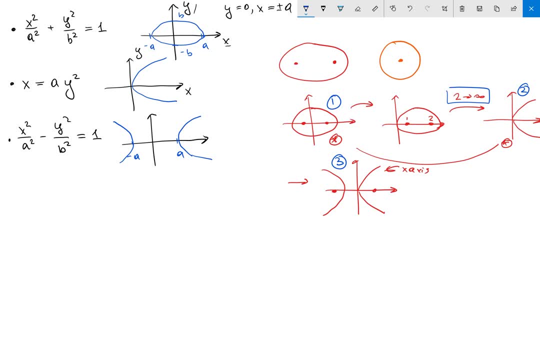 sending our second focus to infinity and sending back to 0. but all these ideas seems a little bit unnatural. so let's actually show you the natural picture why all these three curves are going to be the same, and the idea is really simple. let's talk about 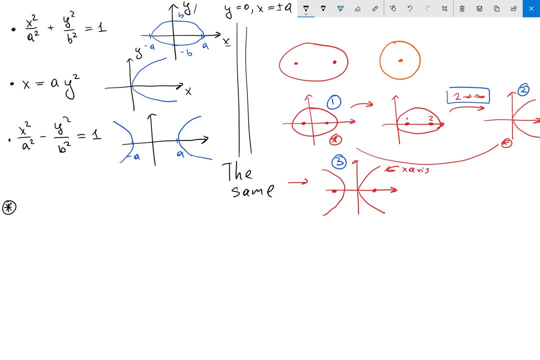 stereographic projection. so the first example that I want to show the stereographic projection for a simple circle. so let's have a circle and let's have x-axis and we can construct stereographic projection by taking the point on the north pole and drawing a line, a straight line that is going to intersect x-axis in. 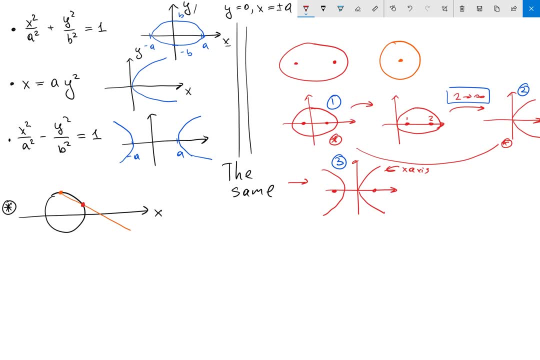 this case, I can see that for every point on my circle, I will get a unique point on my x-axis and the upper half of the circle are going to represent, like this region, another part of the circle like this one are going to represent this region and 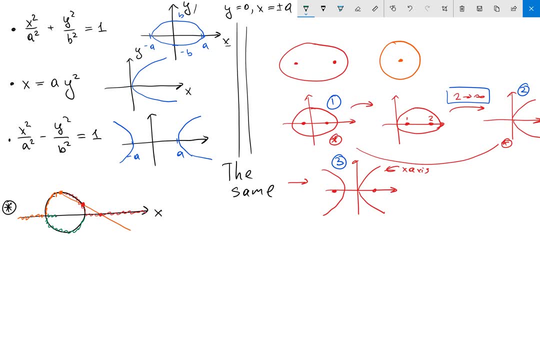 the bottom of the circle are going to represent the inside of my circle. and why is this true? because if I will draw a line, I can see that for this point, I will have this corresponding point on my x-axis. okay, so this is stereographic projection of the circle into x-axis. and let's find the stereographic projection. 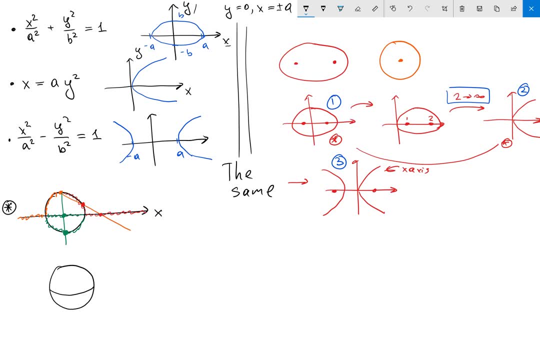 of a sphere, but in this case I will find the stereographic projection of a sphere into the plane. and one thing that I need to mention for my projection of a circle: that I have an infinity point and infinity point. I can see if I will draw my line further. 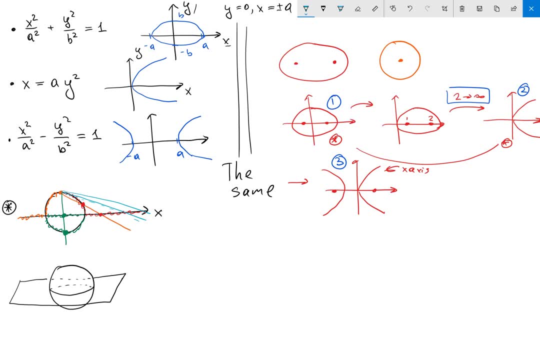 further and further in positive x-direction, like this line, are going to be for the value when x is infinity. so in other words, there is no like such number as infinity. so what I'm going to do, I'm going to draw away this point in North Pole. so I'm saying that s1 without 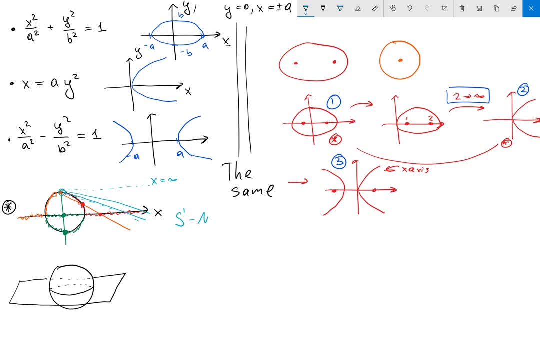 let's say like maybe minus, minus North Pole is going to be homeomorphic to R, but if I'm going to add like a North Pole, it's going to be okay. so just don't want to talk about these details, but let me actually show my first goal. why? an? 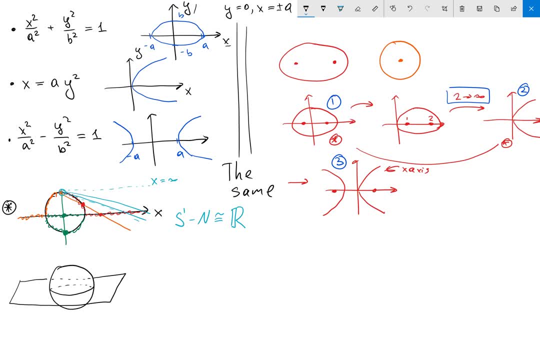 ellipse, parabola and hyperbola is the same curve. so let's think about right now this: geographic projections. so what I will have: I will have my North Pole for circle and then I will intersect my point in my sphere and I will find the corresponding point on my plane. and this: 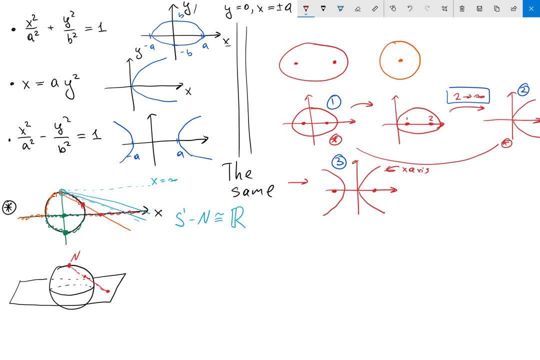 is the graphic projection. so, in the same way as we did for a circle, we can construct this geographic projection of our sphere. and right now let me show you a trick. so let's take our ellipse in R2. in our ellipse in R2, let's say, it looks something like this: 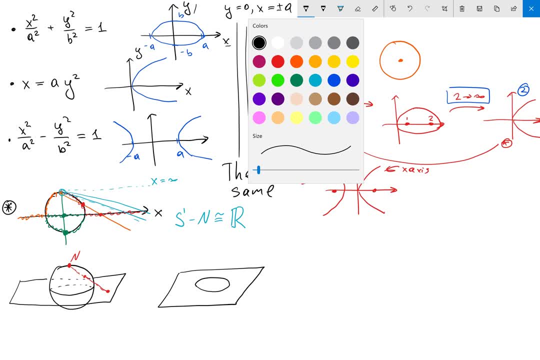 yes, so what I can I do with my sphere? I can do kind of geographic projection on my sphere. it's not really beautiful sphere, but let's do it in this way. so I'm going to do the same geographic projection, but I will go to North. yeah, I. 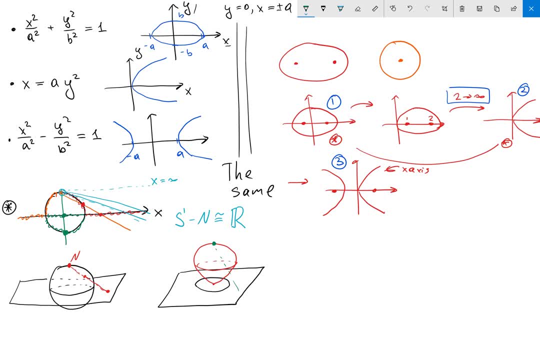 will. I will do the same to represent, but it will go to North Pole. I'm going to send like this, so have this point, this thing, and I can see when my ray is going to intersect this surface like an ellipse. I will get the corresponding picture. I respond: the curve on my sphere, so in other words, my sphere, that looks. 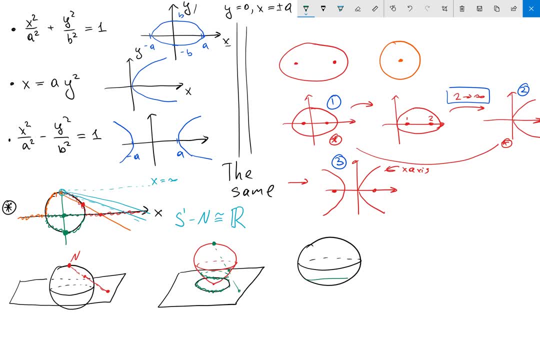 like this and the lips on my sphere is going to look something like this and I will get the corresponding picture. I respond: the curve on my sphere. so, in other words, my sphere is going to look something like this and I will get the corresponding picture. so it's going to be intersection, so it's going to be a curve in my sphere. so when 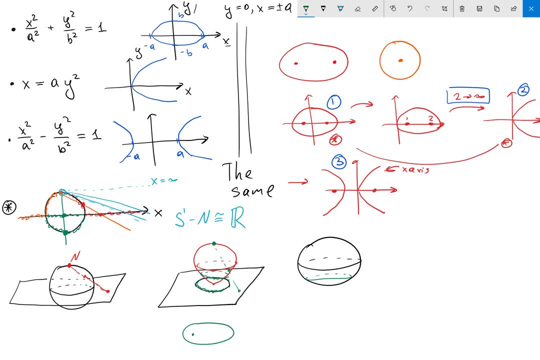 for my in ellipse, which looks like this: I have two focus points, and this focus points is basically saying that I have them over here, this points, and when I have my focus point one, focus point two and then I'm sending two to infinity. it means you just taking this point and 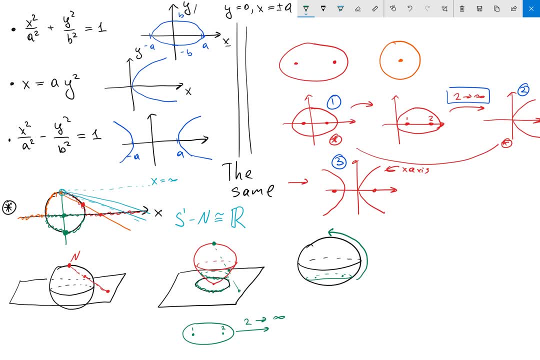 stretching my ellipse to the North Pole. so because this my point, as you remember, this North Pole is my infinity point. so this is this point which is I exclude from my s1. so after I'm going to send my two to infinity, I'm gonna get the 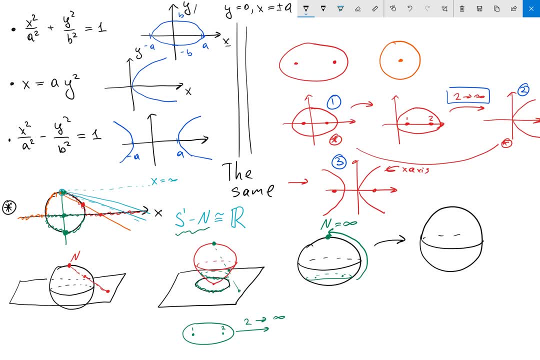 following picture. I will get that how we should draw this correctly and we'll go. I will get something like this and it's going to be lips. so one my foci point is going to be over here and another fucking point is going to be over here. yes, and in this case, like our 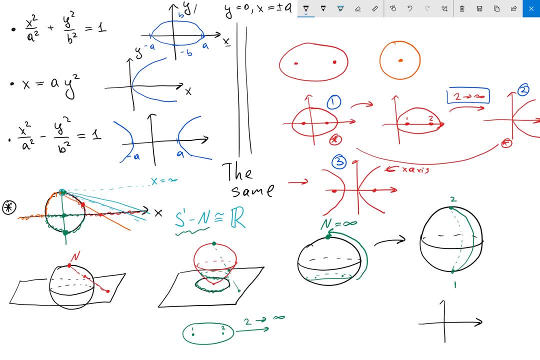 picture in r2. if I'm going to do is to graphic projection. it's going to be that my ellipse is going to looks like this: it's going to be actual parabola you can see, so you can just take this point and you project this point into our team. yes, 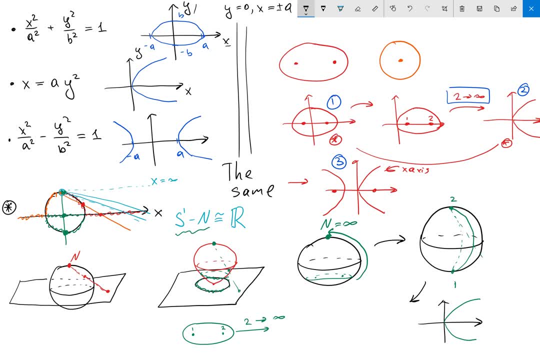 and the last thing, how good I can get a her par bolo. I'm going to come back about what I'm going to do. I'm going to take this point and turn around from other direction. so, in terms of this fear I will have, that my lips is gonna look.